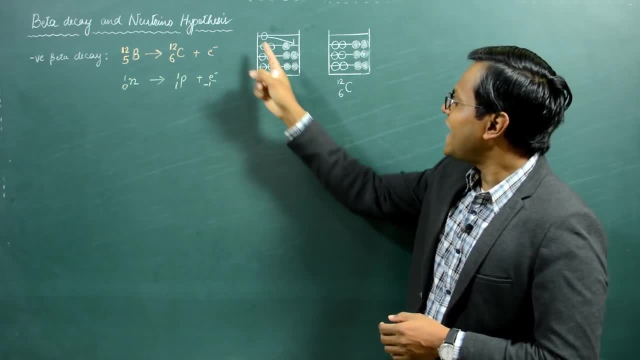 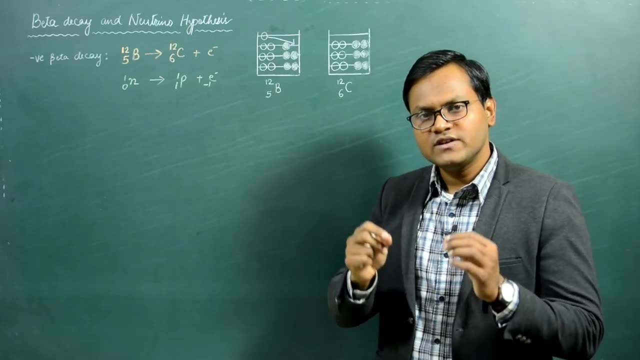 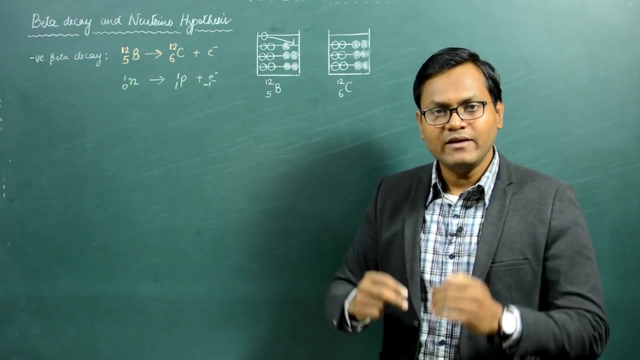 both these two nuclei. So in boron-12 you have five protons and seven neutrons, while in carbon-12 you have six protons and six neutrons. Now, because neutrons and protons are fermions, so no more than two of the same kind of fermion can occupy a given energy level. So basically we 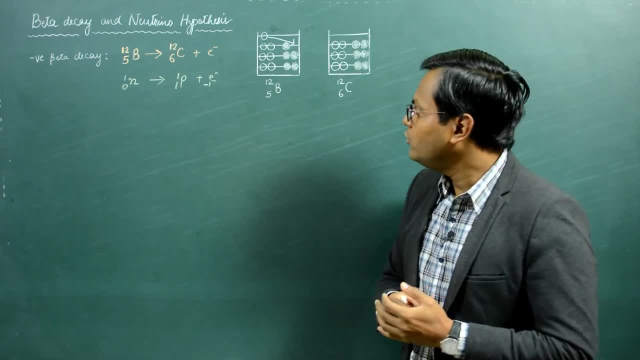 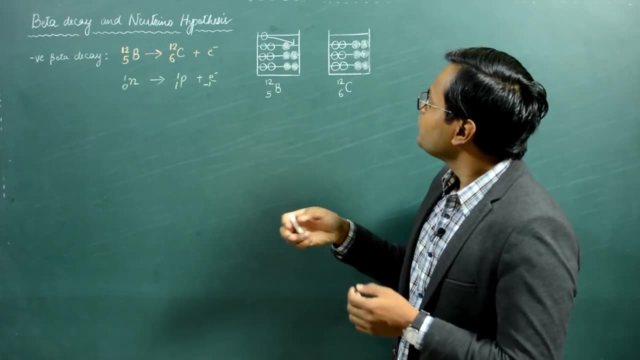 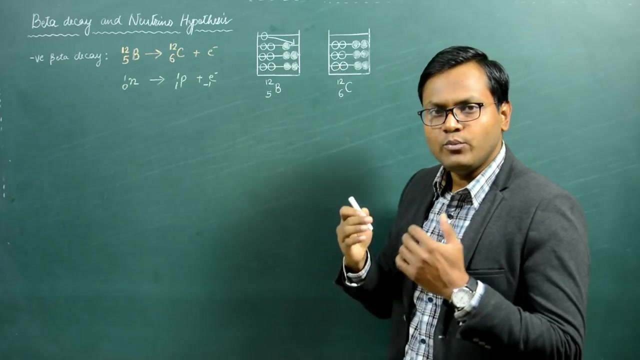 end up getting this kind of energy level diagram for both these two nuclei, Because there are two neutrons which are in excess inside the boron-12 nucleus. you can see here that the nucleus which is occupying the highest energy level, which is this nucleus, is occupying an energy level which 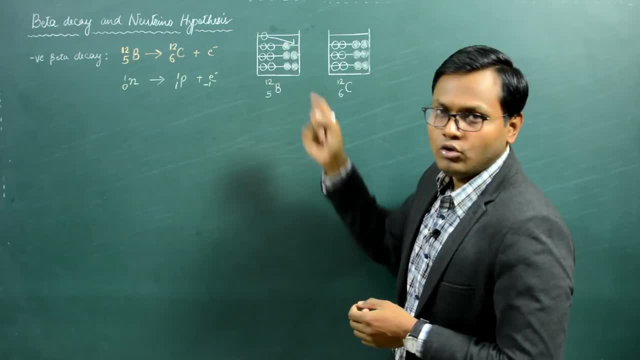 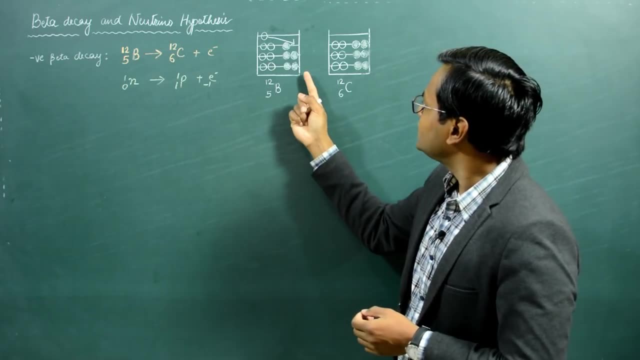 is greater than the energy level of the highest proton. So the neutron is occupying the first, second, third, fourth energy level, while the highest occupying proton is occupying the first, second, third energy level. So the neutron is occupying energy level which is greater than 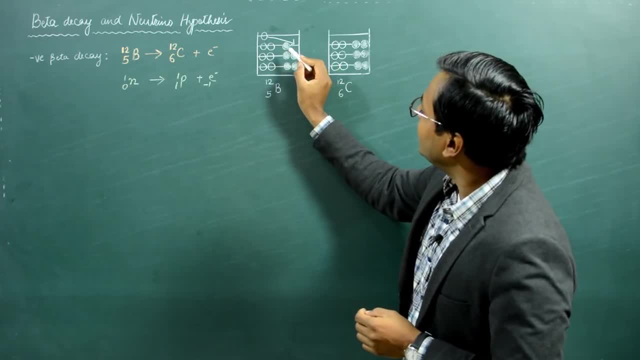 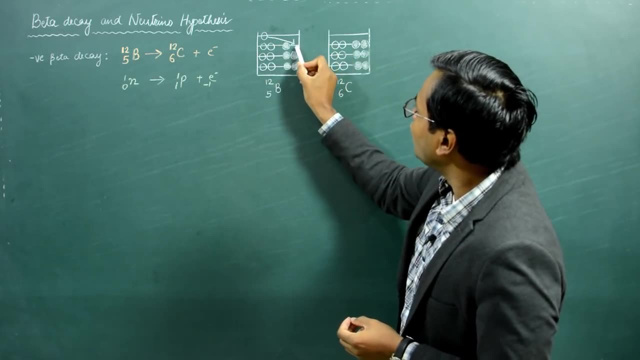 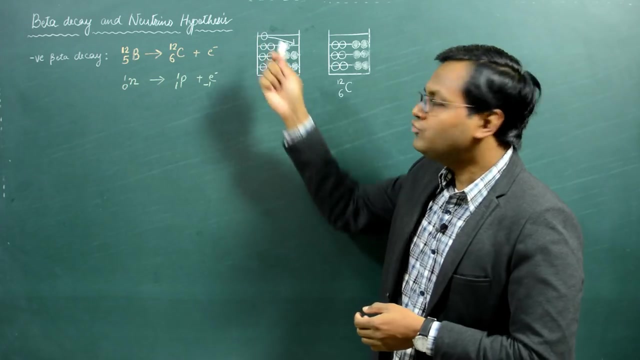 the highest occupying proton and there is also a vacancy in the highest proton energy level. So if somehow this neutron gets converted to a proton, then this new proton will occupy an energy level which is lesser than the neutron energy level, thereby decreasing the overall energy configuration. 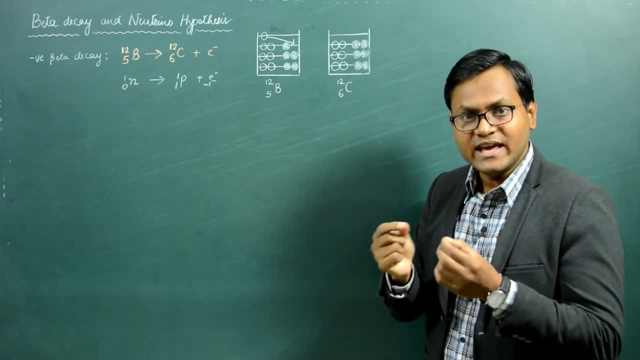 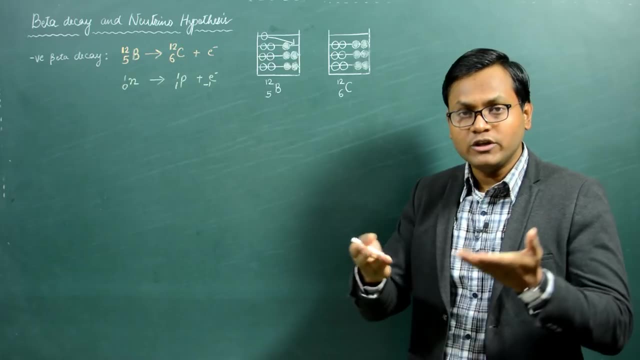 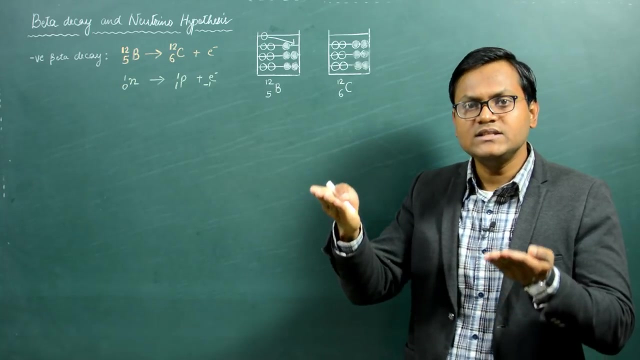 Thus we end up getting a carbon-12 which has less energy and more stability. So this is what happens in a beta decay process: Whenever a neutron or a proton is occupying a higher energy level because they are in excess, they might get converted to the other kind of a particle, thereby decreasing the overall energy of the system and increasing 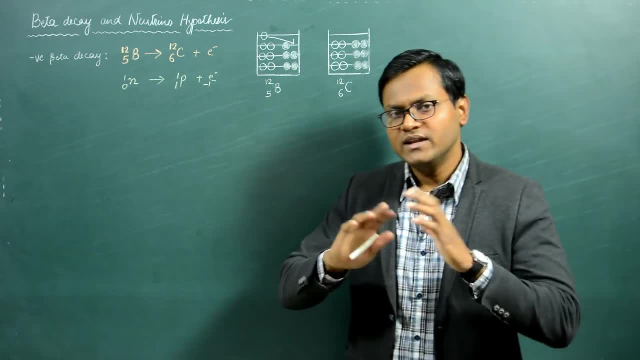 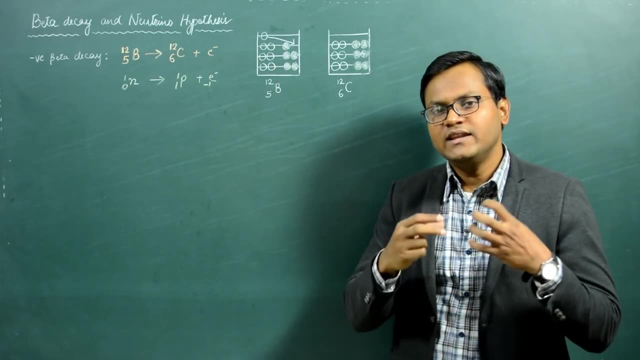 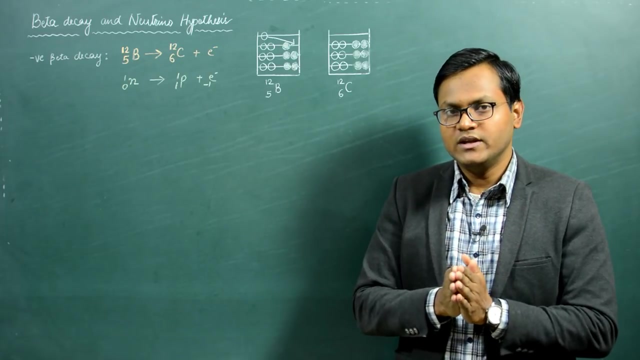 the stability of the nuclear configuration. This is why beta decay reactions happen in the first place. Now, before talking about the different kinds of beta decay processes which are seen in nature, we need to discuss a very interesting and a very important historical development which is associated with the beta decay process, which 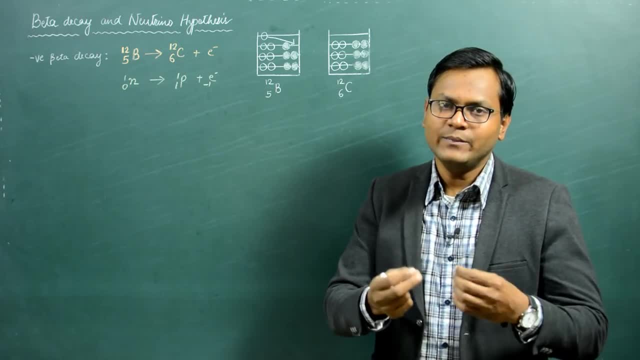 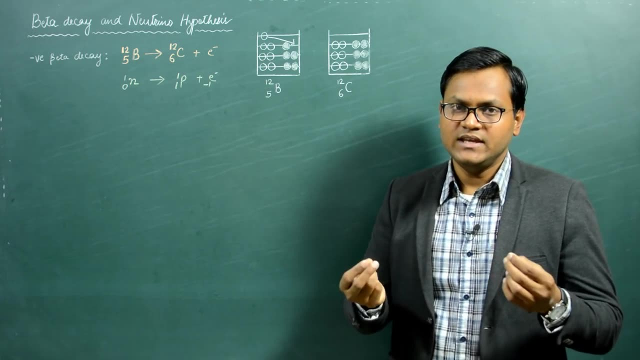 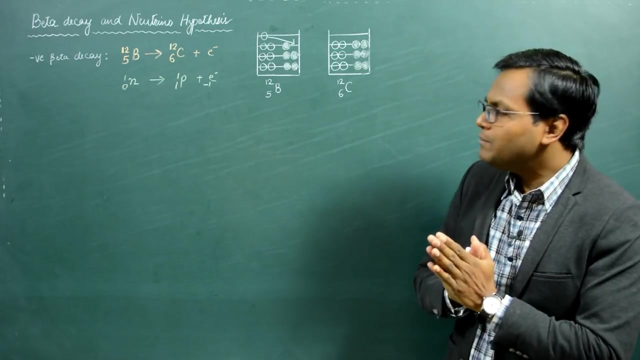 has to do with the prediction of a very new fundamental elementary particle. This is known as the neutrino hypothesis. So studying the experimental aspects of beta decay led scientists to predict a completely new fundamental elementary particle. How it happened So? it happened by looking at the seemingly violation of certain kinds of physical laws which were taking place. 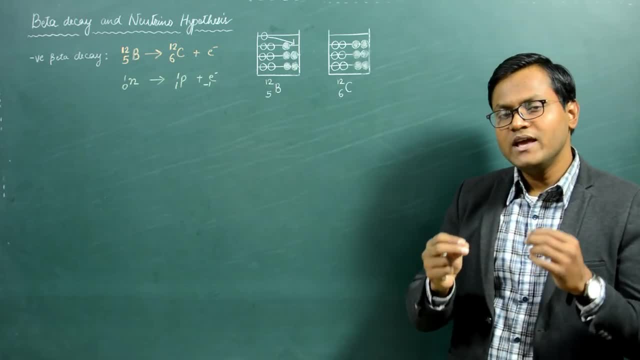 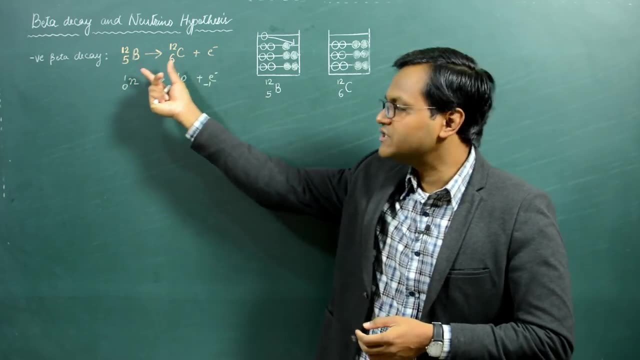 in the nuclear system. So if you look at the kinetic energy of an electron, it was found that theoretically we can calculate the kinetic energy of an electron by looking at the disintegration energy which is associated with a given nuclear reaction. So whenever a nuclear reaction takes, 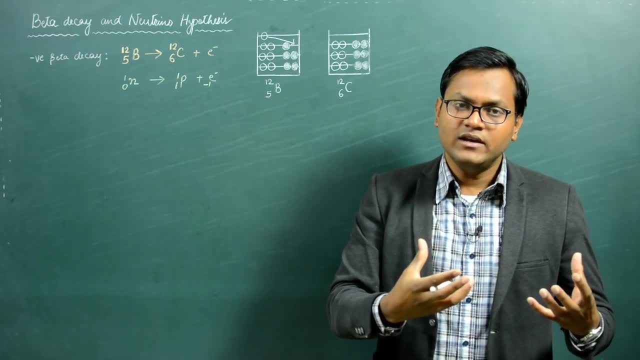 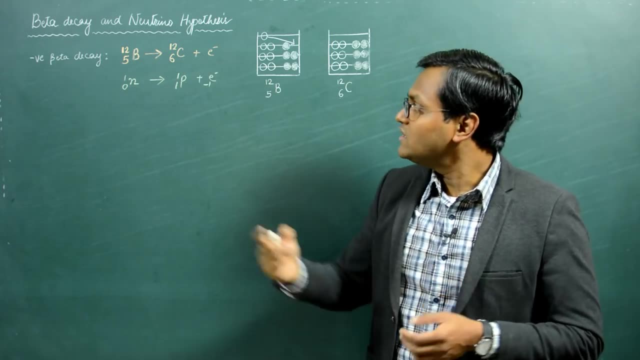 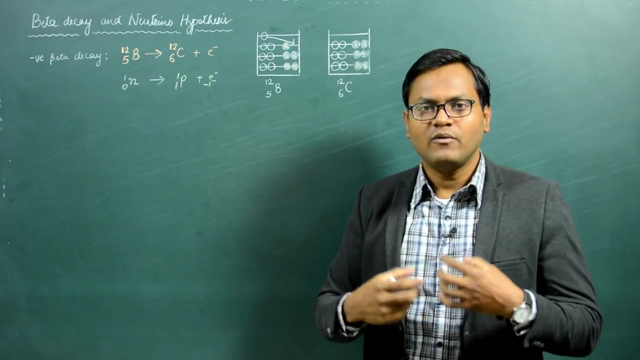 place some amount of energy is released. We can predict the energy released by looking at the mass defect and from that energy we can also predict the kinetic energy of the emitted particle. because daughter nuclei is so massive, the vast amount of disintegration energy is carried off by the electron in the form of kinetic energy. So we can theoretically predict. 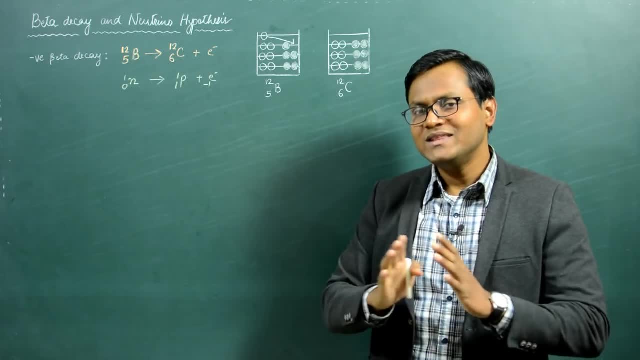 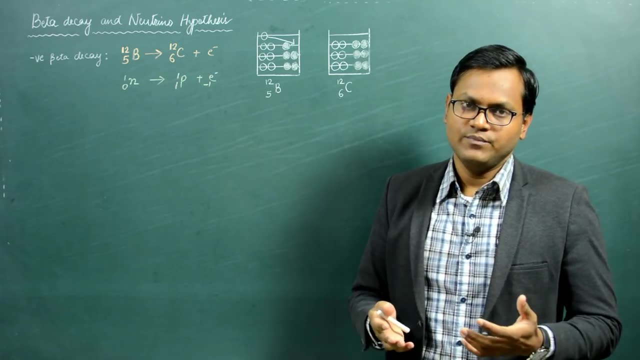 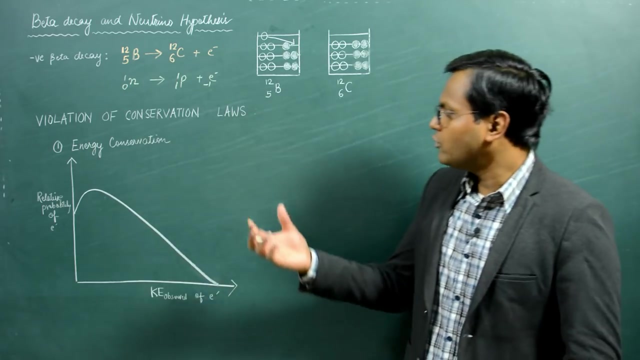 the kinetic energy of the electron. However, experimentally, when the kinetic energy of the electron was studied, it was found that the kinetic energy of the electron had a continuous distribution. We can look at this from the specific graph. So this graph here basically tells us the energy distribution of the electrons when we study a same nuclear reaction over and. 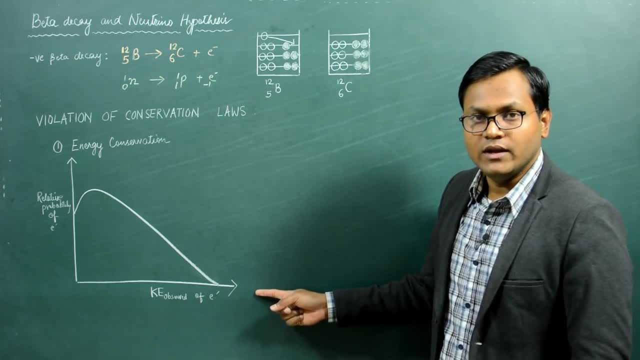 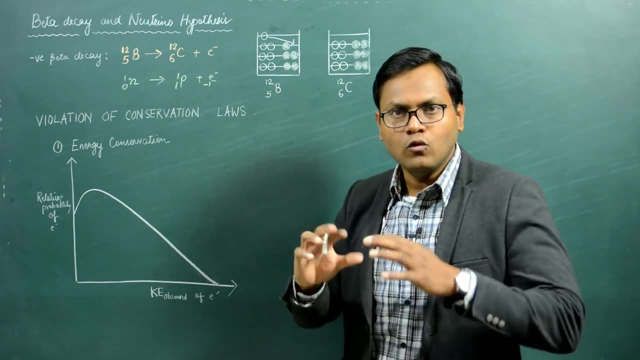 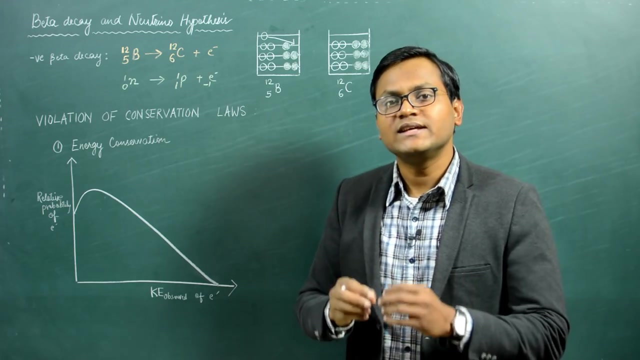 over again. So the x-axis represents the kinetic energy of the electrons and the y-axis represents the relative probability of the electrons. So if you study the same nuclear reaction over and, over and over again, then the electrons seem to have kinetic energy which is not fixed, but rather it. 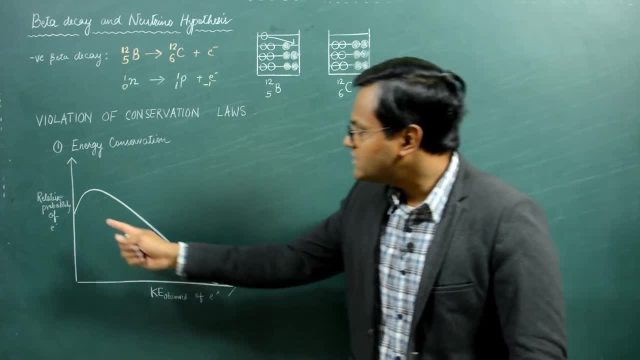 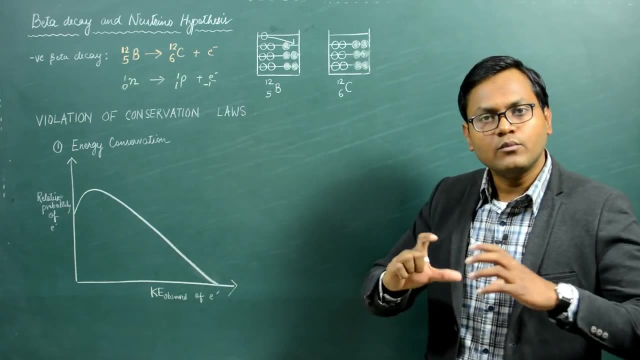 has a continuous distribution. In some cases the electrons are seen to have zero kinetic energy. in some cases- a very rare cases- the electron is seen to have maximum kinetic energy. but for most of the cases the electrons fell in a continuous distribution. Now, beta decay reactions, just like 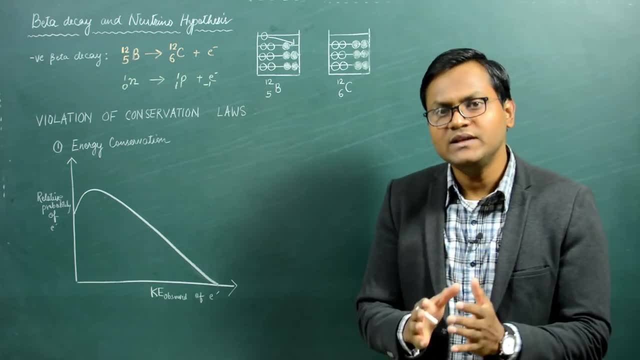 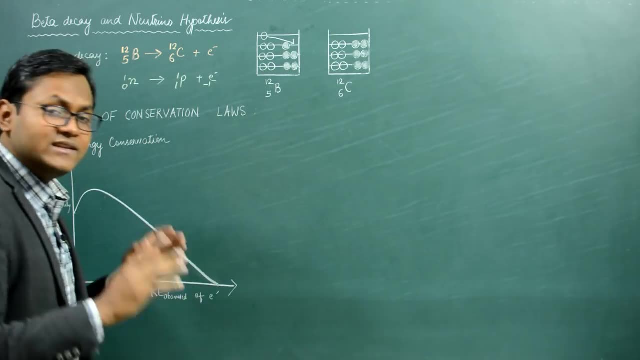 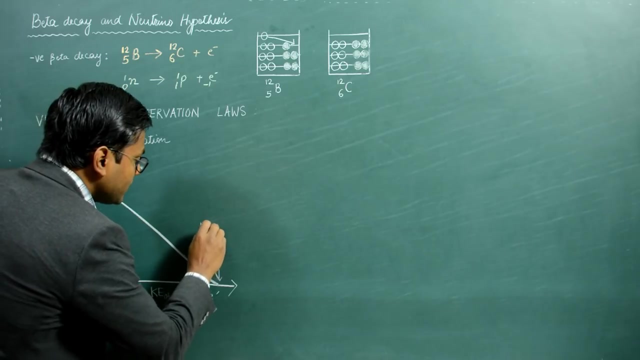 alpha decay reactions are monokinetic in nature. that means the kinetic energy of the emitted particles should have a fixed value which can be theoretically calculated, and in our case the beta decay should emit a kinetic energy of an alpha particle, which is this. So this is the 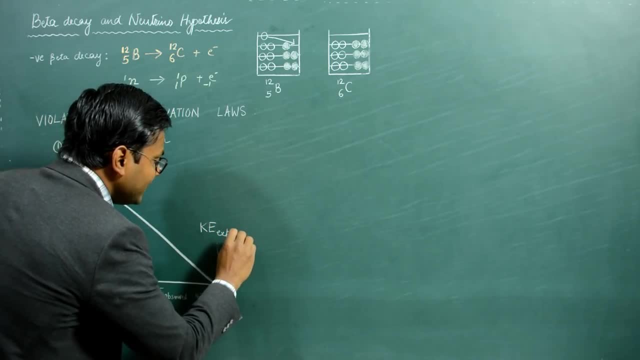 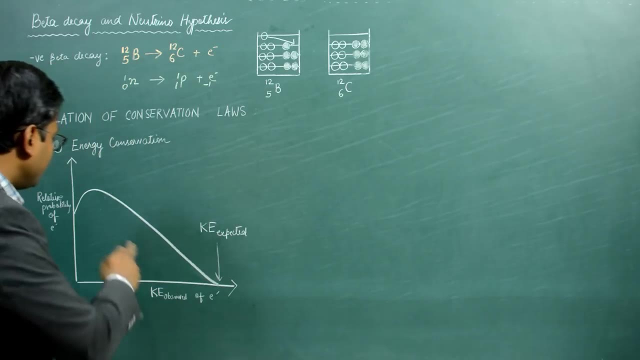 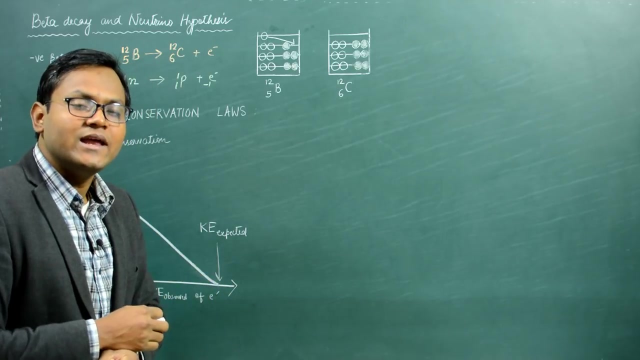 expected kinetic energy based upon theoretical calculations. So this is the expected kinetic energy of the electron. however, the experimentally observed kinetic energies fell in a continuous range. So let's suppose that you perform a nuclear reaction and then you look at the energy of the electron which is emitted and you find that maybe the energy of the electron emitted lies somewhere. 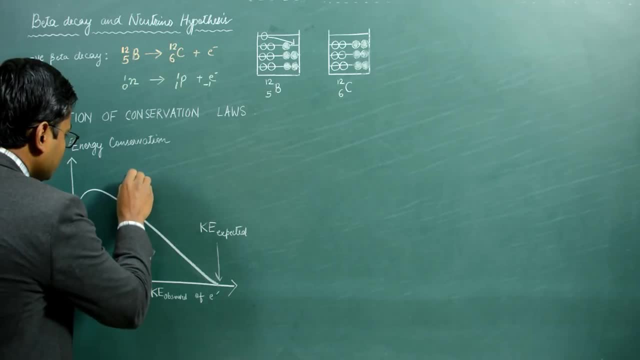 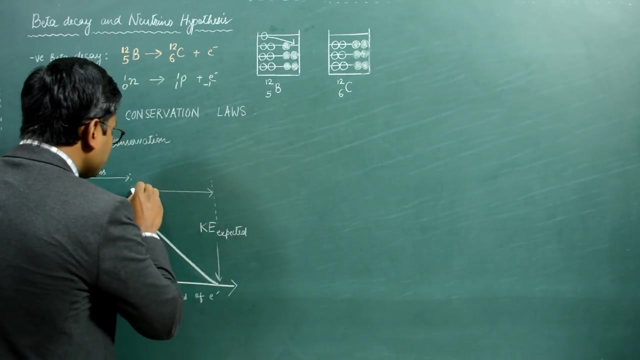 let's suppose here, all right, if this is the case, so this is basically the energy of the electron which is experimentally observed in your case, then what happened to the rest of this energy? So where is the rest of the energy gone? So this is a basically. 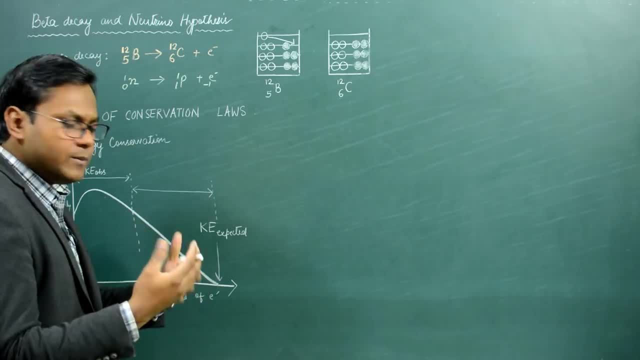 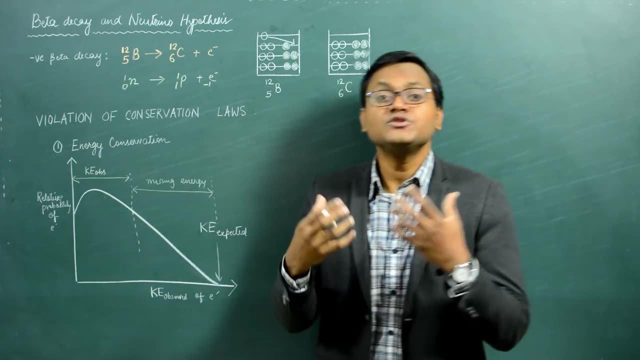 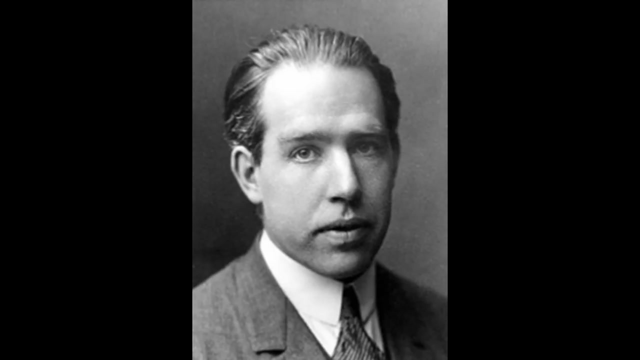 a very puzzling aspect when you look at the experimental data, that some of the energy is missing. So where did this missing energy go? There was no explanation. in fact, this kind of a data was so much puzzling that the very famous scientist, Niels Bohr, who gave the Bohr model of 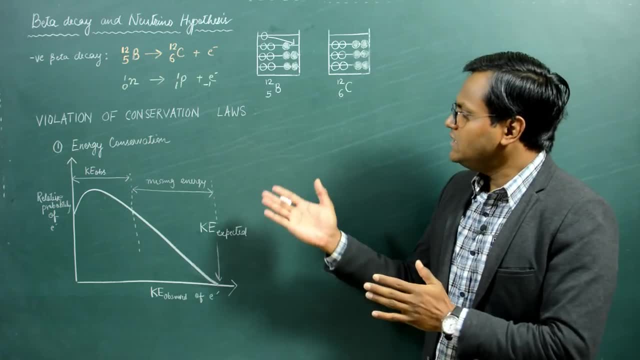 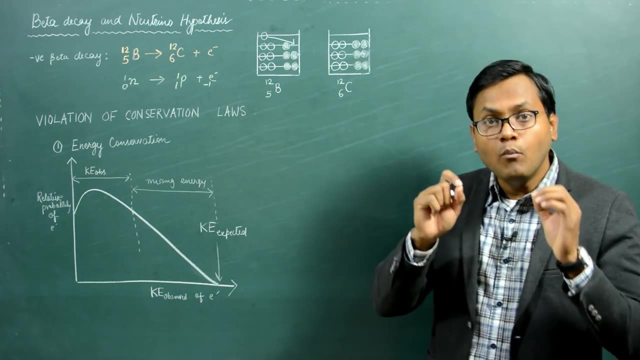 atom suggested that maybe the beta decay is violating the conservation law of energy. and not just this, even the conservation of momentum was seeming to have a negative effect on the energy, And it is seemingly violated in this process. So if you look at the directions in which these 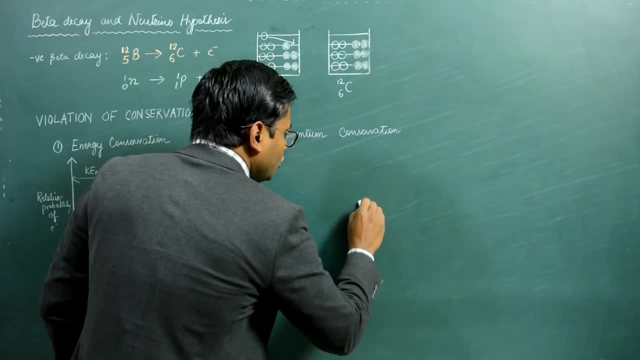 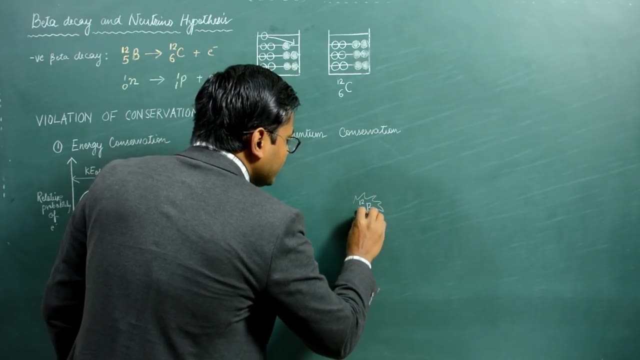 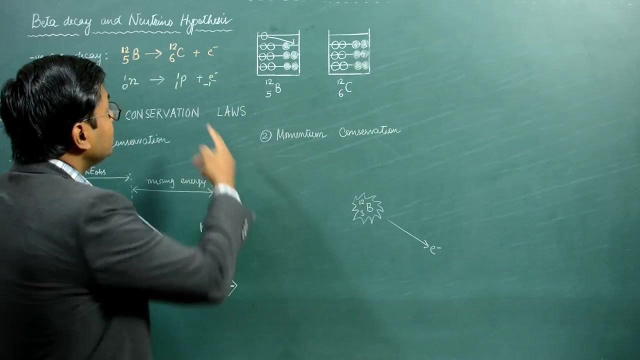 particles are being emitted. so let's suppose that you have a boron-12 before undergoing radioactive decay process and suddenly this boron-12 undergoes a radioactive decay process. then now, suddenly you have an electron which is emitted in this kind of a process and a recoining daughter nuclei which is the carbon-12.. When you study the directions in 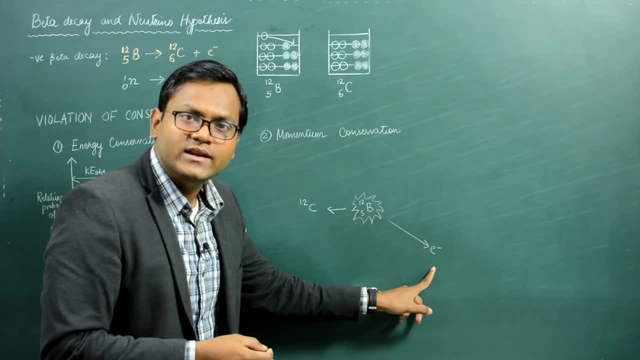 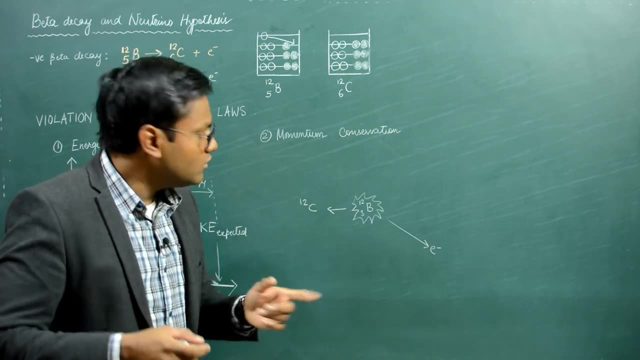 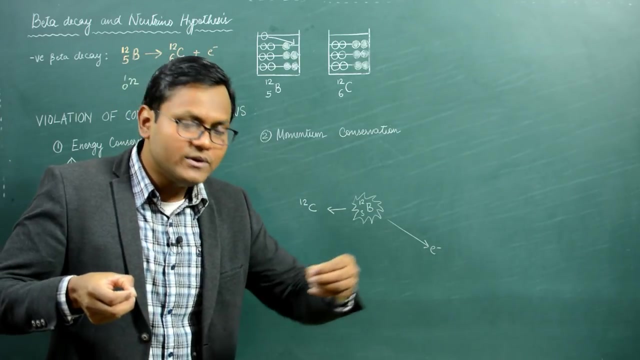 which these particles are emitted, then it is seen that the electron is emitted in a direction which is not exactly opposite to the recoil of the daughter nuclei. This is confusing because if there are two particles which are involved, then conservation of linear momentum tells us that the recoiling particle and the emitted electron should move exactly in opposite. 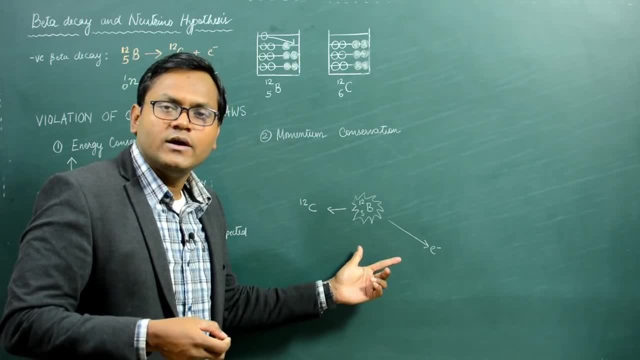 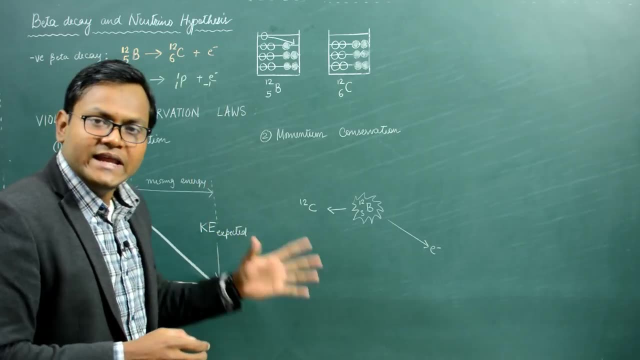 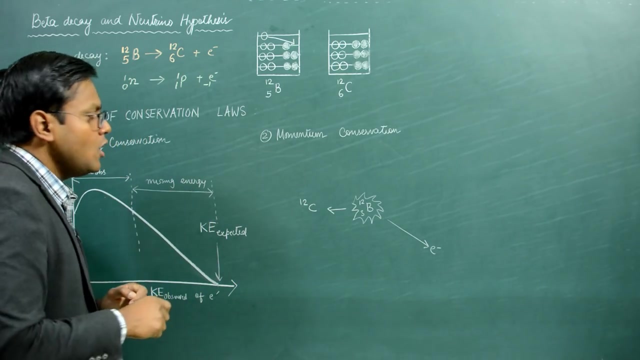 directions to conserve linear momentum. This shot of a recoil does not conserve linear momentum, so it was even suggested that maybe k was violating the conservation of momentum principle. It did not stop here. There is a discrepancy when you also look at the spin of the particles involved. When you look at the particles, 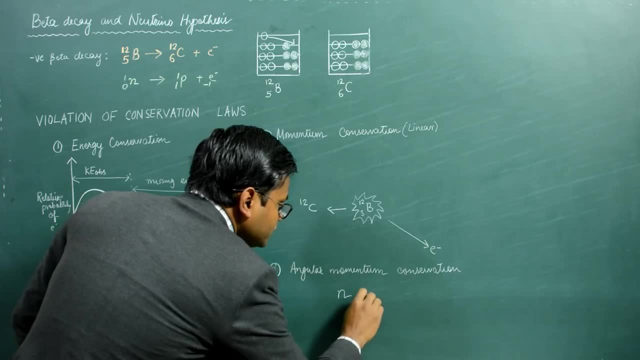 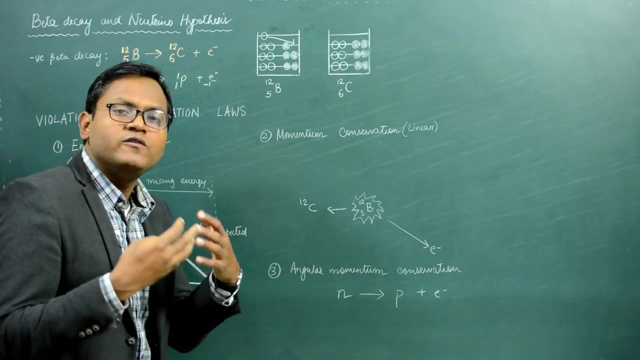 which are involved here. so in this case you have a neutron which is becoming a proton and also leading to the emission of an electron. in the first place, these particles are all fermions. That means a neutron has a spin of half, proton also has a spin of half. 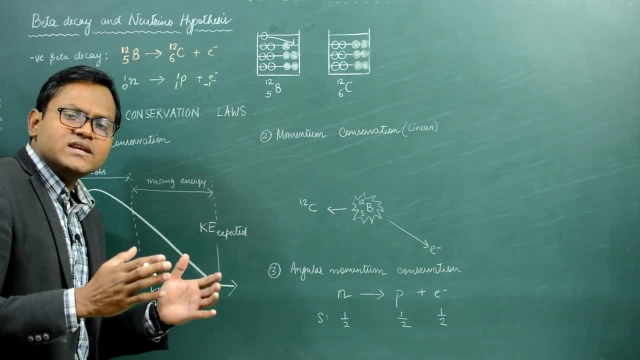 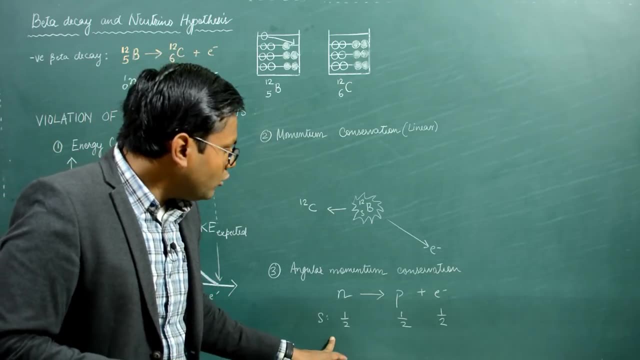 An electron also has a spin of half. This is violating the conservation of spin angular momentum. Why? Because one spin half particle cannot lead to the creation of two spin half particles. The spin in the left hand side and the right hand side are not balanced, and because 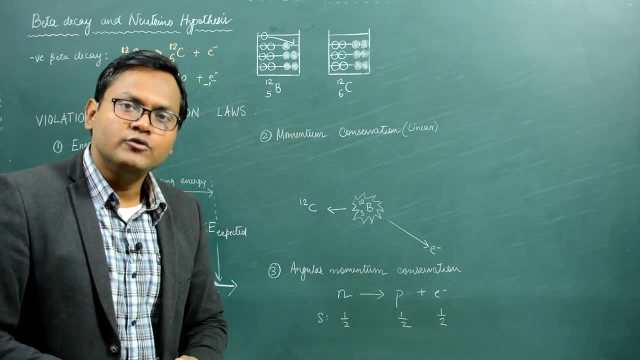 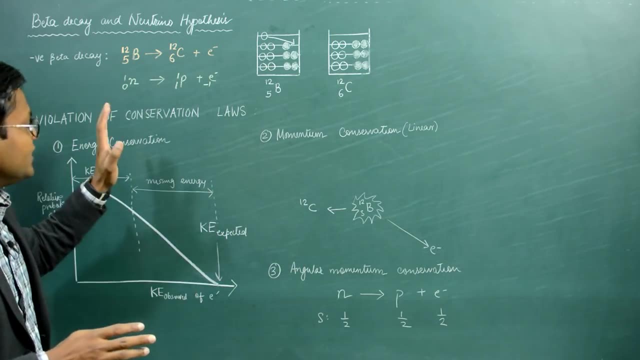 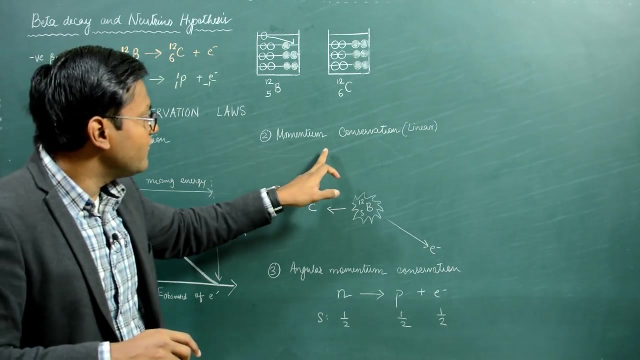 spin directly relates to the spin angular momentum of those particles. the angular momentum is in this reaction is not conserved. So, as you can see here, the experimental data associated with beta decay suggested the violation of conservation of energy principle, the conservation of linear momentum principle and the conservation of angular momentum principle. However it did. 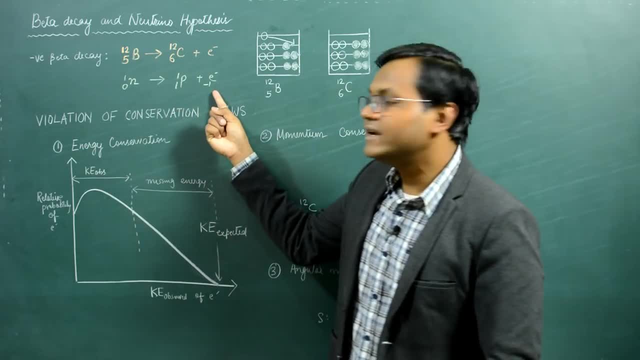 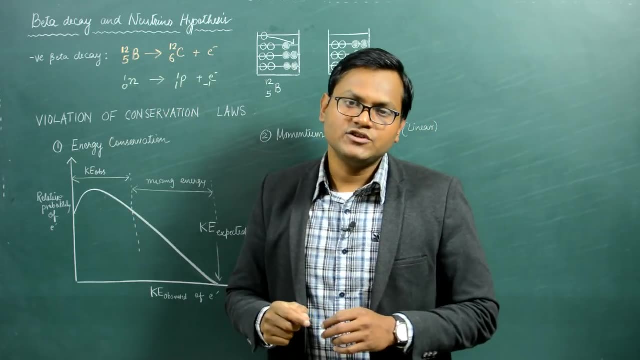 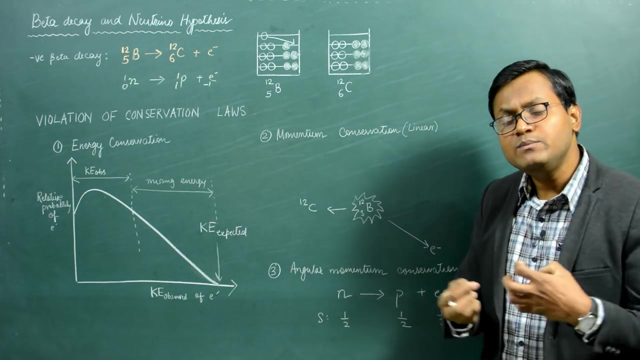 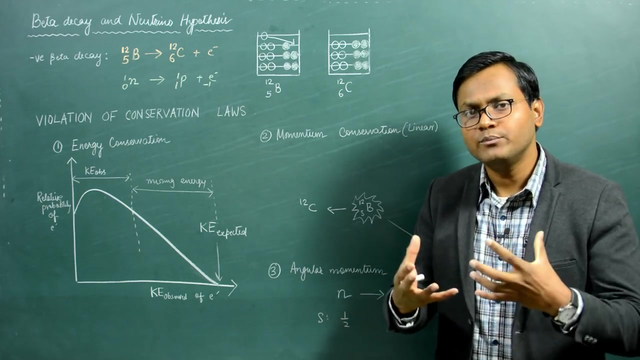 not violate the conservation of charge, because electron is negatively charged, proton is positively charged and the neutron is neutral. It maintained the conservation of charge here. So what is happening except charge being conserved? the other important physical laws were seemingly violated in this kind of a beta decay reaction. it was first suggested by Wolfgang Pauli in 1931. 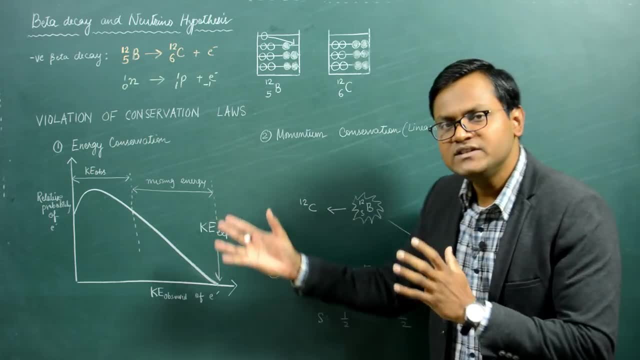 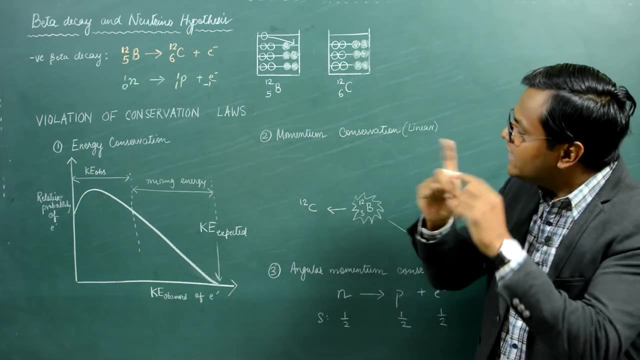 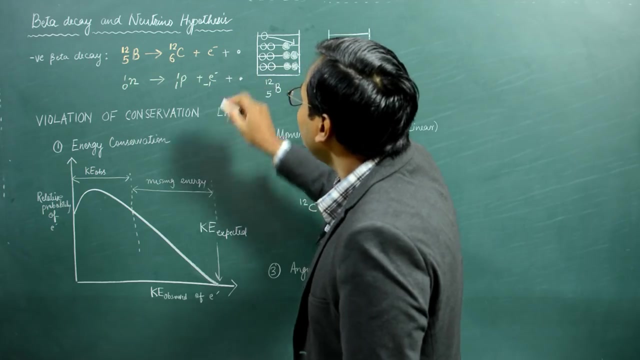 that we can explain the seemingly violation of these important physical laws by introducing another particle in this given reaction. If we assume that there is another particle which is also emitted in this kind of a nuclear reaction, then we can explain why these violations are seen to happen. So if we have a particle in which the charge is conserved, the duration of the reaction, 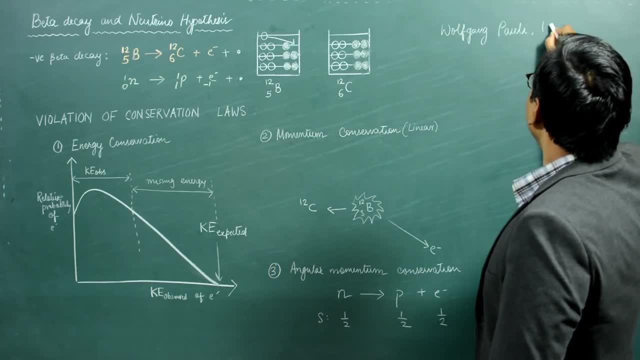 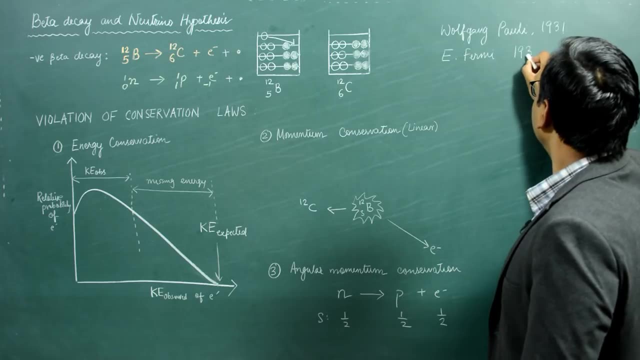 The transition and the detection time are considered to be not impact to the state of the electron. So if we So, it was first Wolfgang Pauli in 1931 who suggested this kind of a particle, and later on Enrico Fermi in 1934 who took this idea forward. and they suggested that because charge. 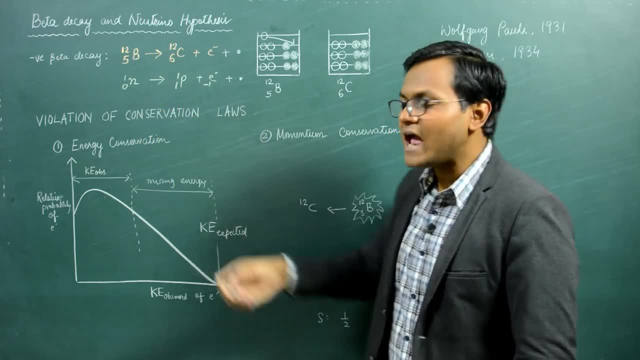 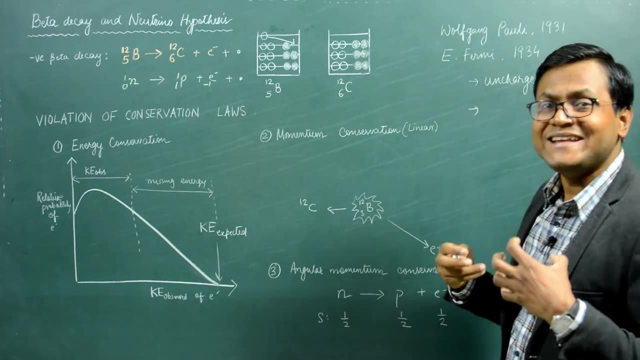 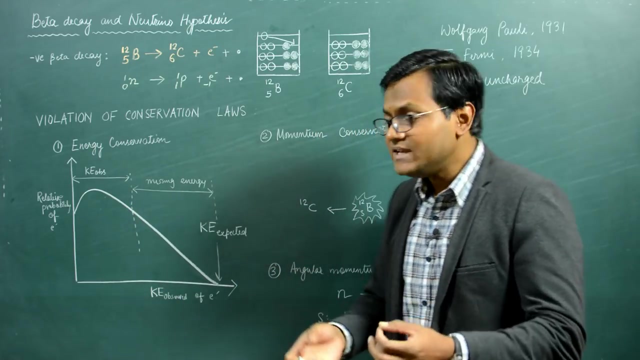 conservation is not violated. charge is conserved in this reaction. So whatever this particle is should be uncharged in nature. It should also have a tiny mass, because this particle is basically taking the total amount of energy from an electron and since electrons are very light, this kind of a particle should.